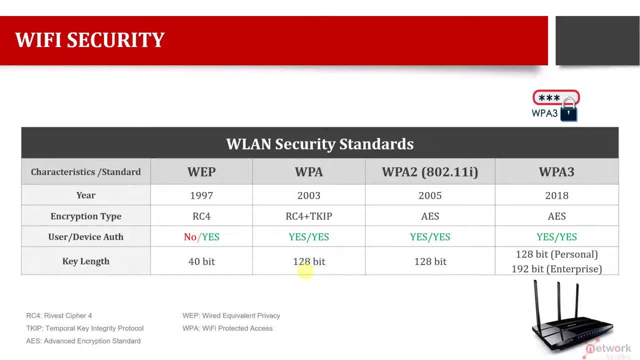 But soon we found security flaws in that one as well, And it was not secured from hackers. That's why we had to come with a new standard called WPA2. It came in 2005 and it supported AES type of encryption, which was advanced encryption standard. 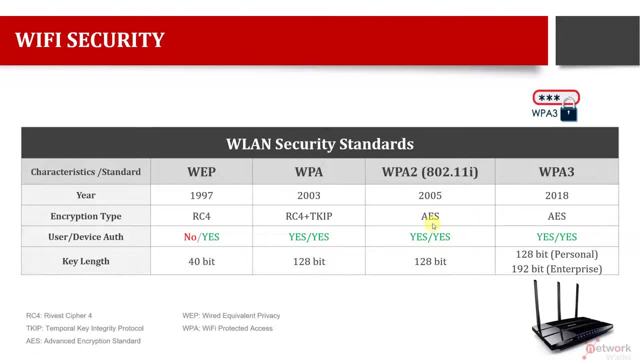 So it's a new and more advanced. So, even as of today, we are using AES. if you go to homeland security department website in America and go to the Wi-Fi and security and online security standards, you will find find that the recommended encryption method is AES, even by US government. 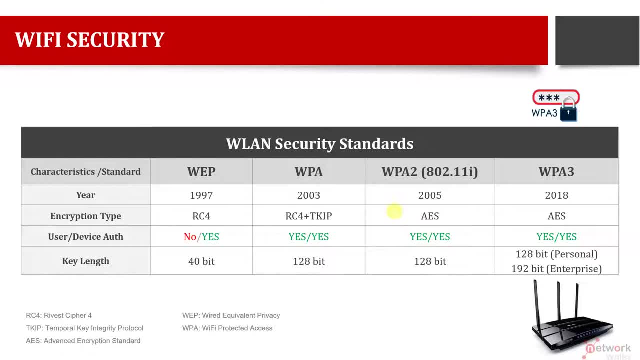 So it is the most advanced method at the moment. It supports WPA2, supports user and device authentication as well, and it gives us two profiles: personal and enterprise. Its key length was also 128.. Then recently, in 2018, we came to find WPA3 encryption and security method as well on 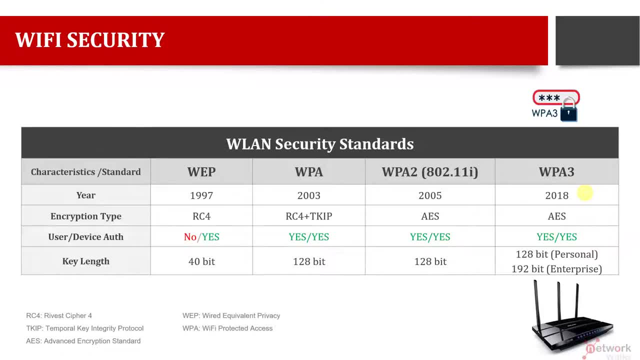 most of the advanced routers but as of today you might not see many routers with WPA3 because it is still in, we can say, in Upgradation or still in integration phase. So usually we find maximum WPA2.. It also WPA3 is available. 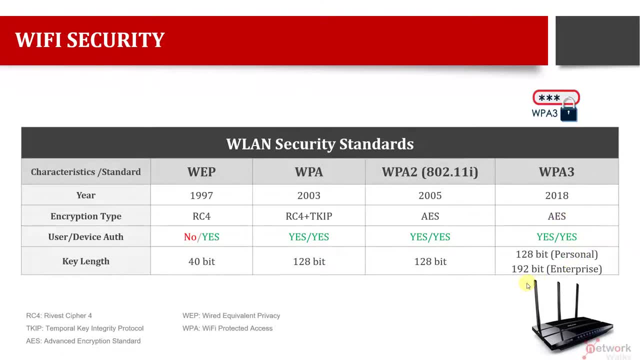 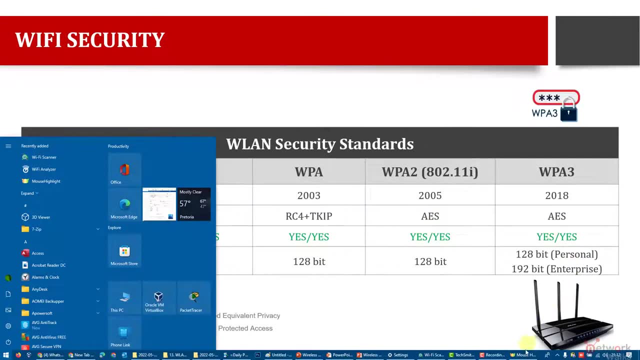 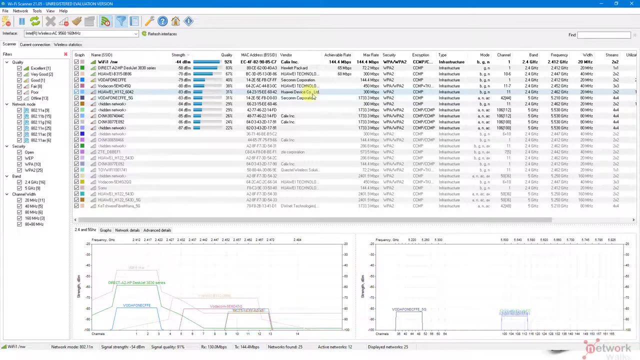 It is also based on AES encryption and it gives a better key length of 192.. So these are some of the security standards. Now let me log into my Wi-Fi and then we can see from the Wi-Fi scanner that which encryption method do we find practically? 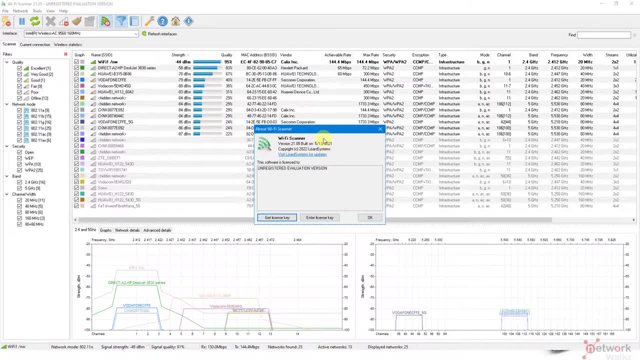 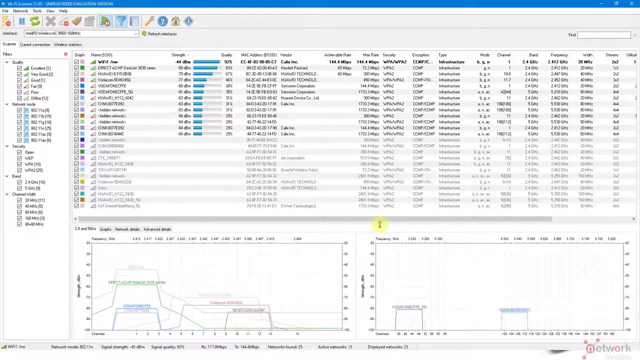 So I'm here on this software. This is called as Wi-Fi scanner. I'm using version 21.05.. If you guys want, you can also Download install. it's a free utility for Wi-Fi analysis, right? It is equally valid for 5 GHz and 2.4 GHz bands. 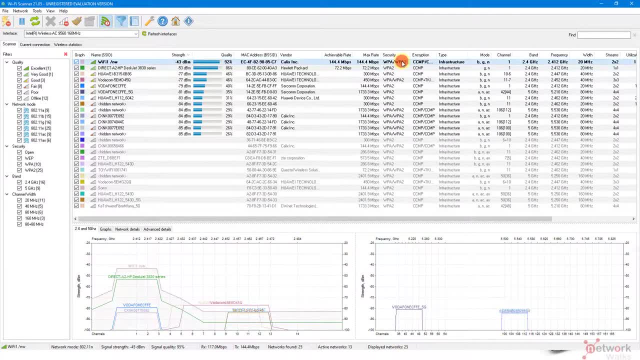 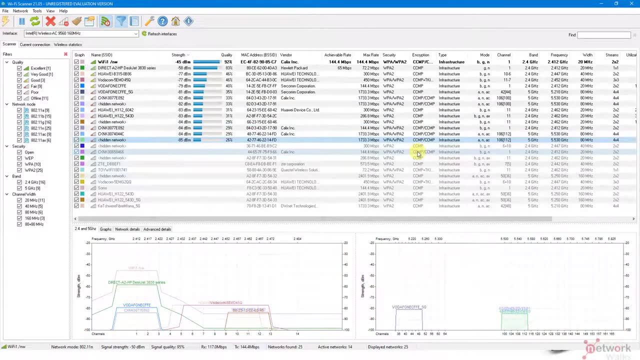 So here we can see different methods, sorry, different Wi-Fi, and most of the Wi-Fi they are giving us WPA2 or WPA, WPA2, mixed mode. Mixed mode means it automatically select. if it's an old type of device doesn't support WPA2, so it will switch to WPA normal. 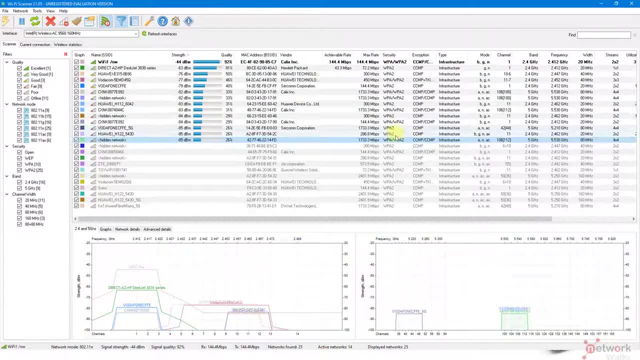 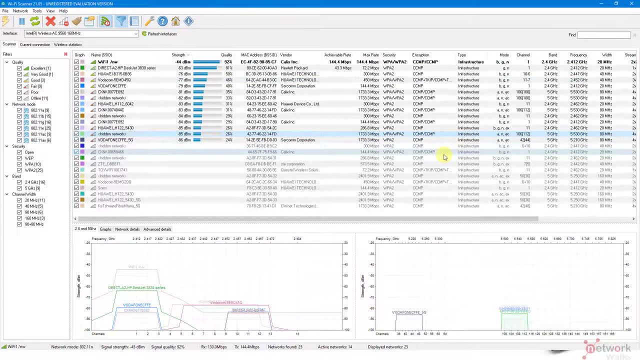 Okay, So these are security methods and the encryptions which they are supporting. they are CCMP, TKIP, all those what I have explained previously and other parameters are there. We can also add and remove columns from here, if you want to add this WPS. 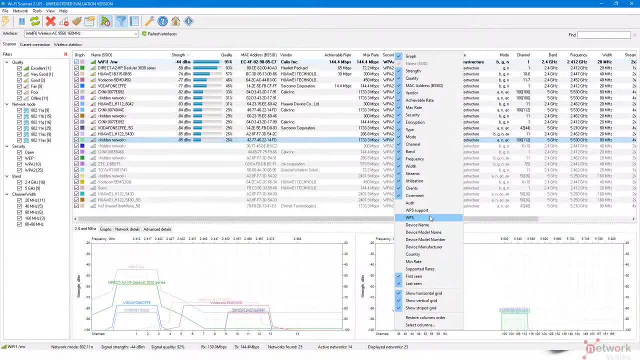 This is a physical button. This is also another security method. we can say: sometime when you are a non-technical person, you can just push a button on your Wi-Fi router. for example, when you want to connect printer, They have a WPS button. just press the button on printer and on the Wi-Fi router and they 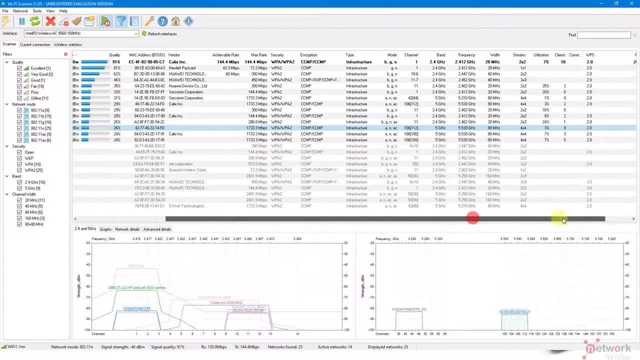 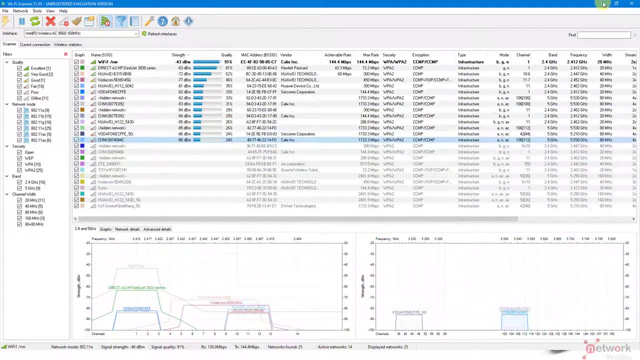 will connect without any password, So we can see which devices are supporting these which are not supporting. So this is how it looks in reality. practically you guys can also verify. So these are some wireless LAN security standards. 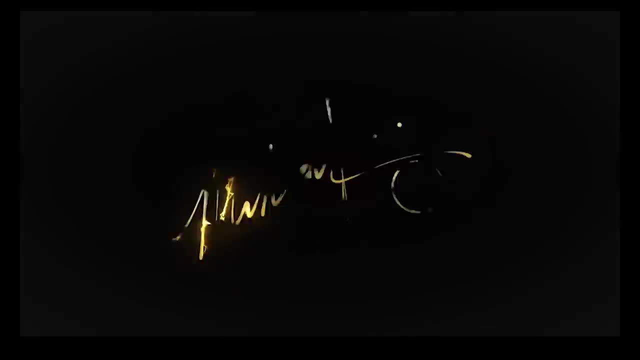 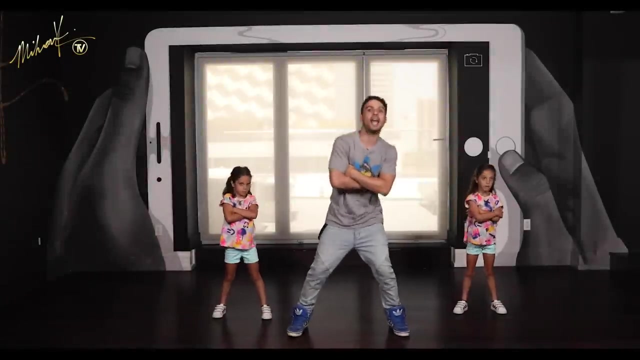 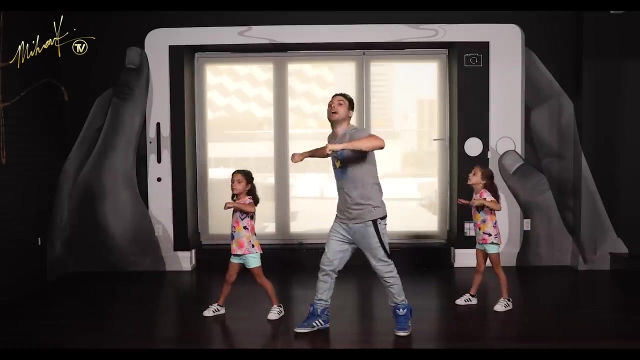 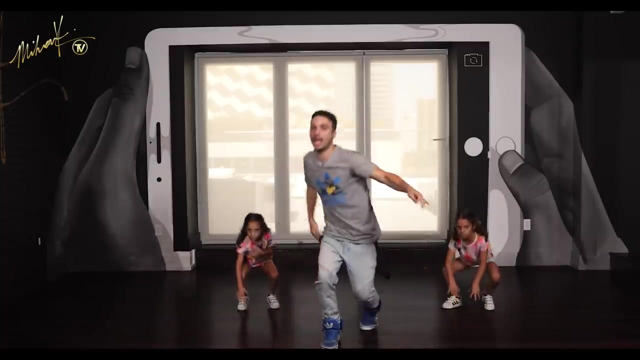 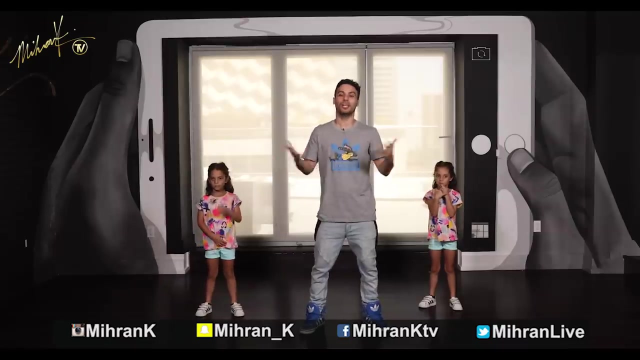 Hey guys, welcome back to another tutorial. My name is Miron Kirakosian. Today we decided to do something a little different. I have my daughters here. They decided to join me in today's tutorial. This is Sophia. Say hi, Sophia.